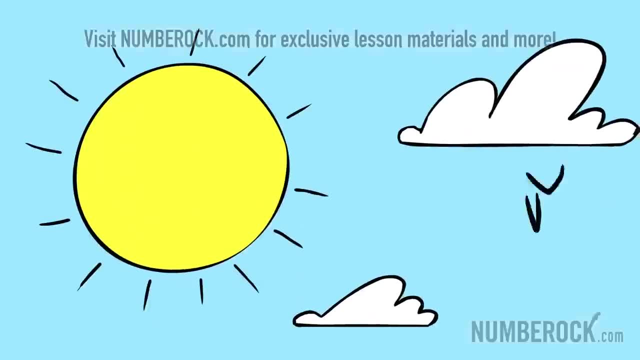 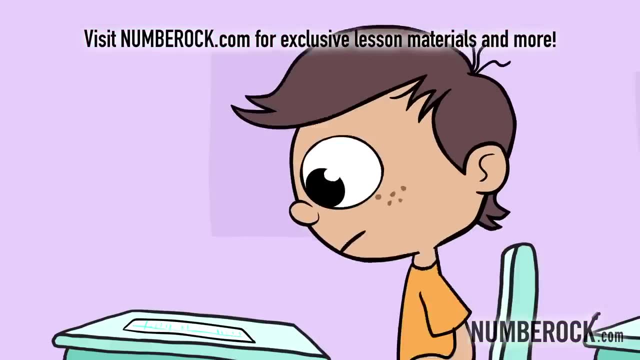 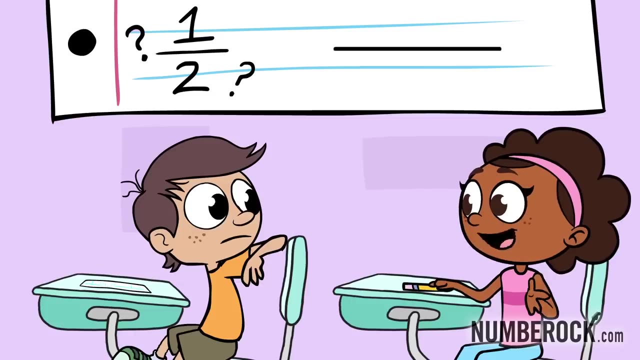 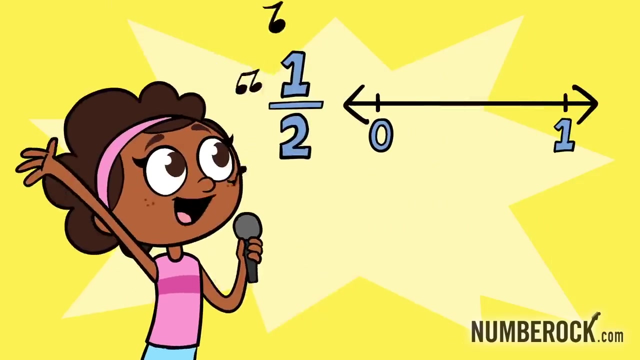 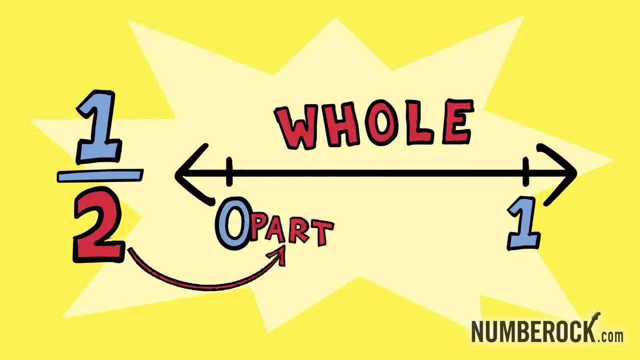 I asked my friend if she could help me find where to write one half on the number line. She said: first draw a line with two arrows, Then she sang a song. here's how it goes: Zero to one is the whole that we split apart. The denominator tells us into how many parts. 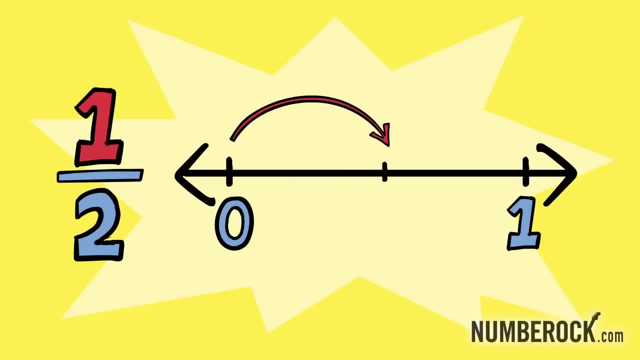 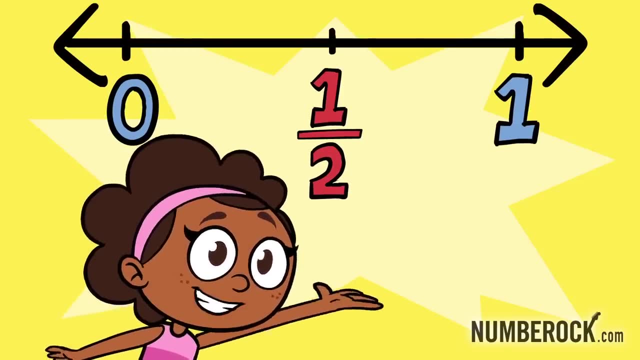 Make a line that starts from zero to the first mark, And one half is what you'll find when you get that far. My stuffed animal can't talk, but I thought I heard Hey Ben on the number line. where's one third? 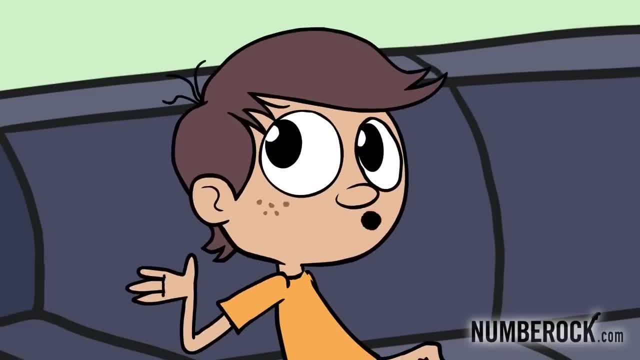 I said: first draw a line with two arrows. Then she sang a song. here's how it goes. Hey, Ben, on the number line, where's one third? I said: first draw a line with two arrows And hey, I know a cool tune. Here's how it goes. 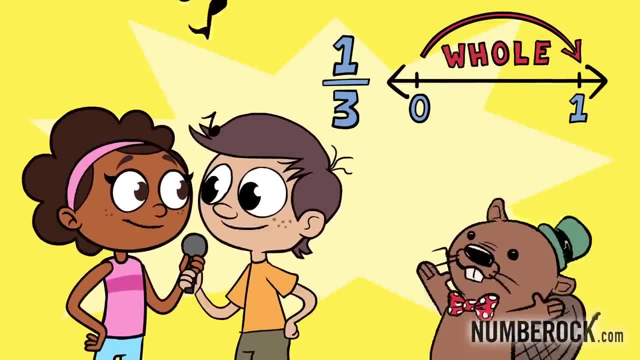 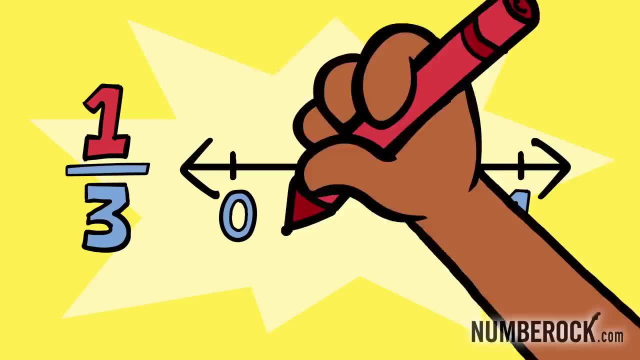 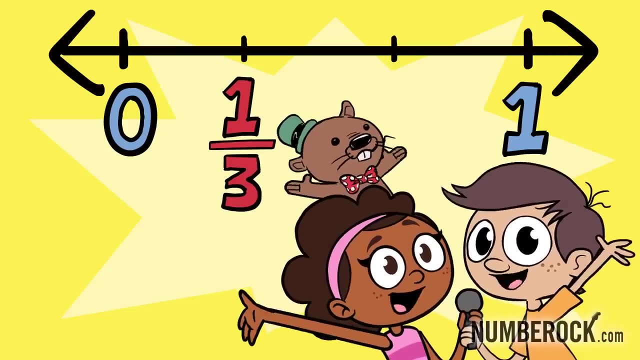 Zero to one is the whole that we split apart. The denominator tells us into how many parts Make a line that starts from zero to the first mark, And one third is what you'll find when you get that far. Then I texted my friend what's to be done. 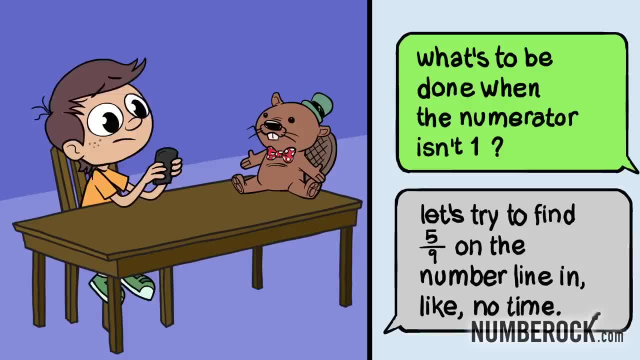 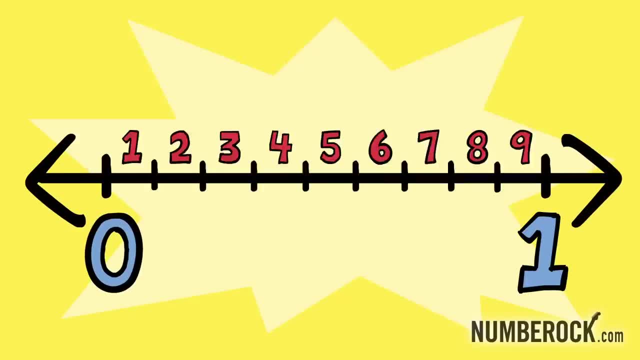 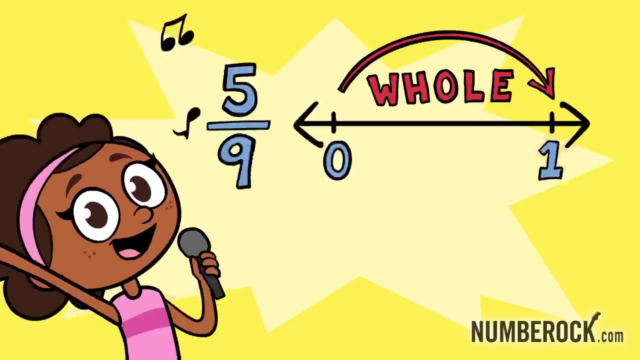 to be done when the numerator isn't one. she said: let's try to find five over nine on the number line in like no time. simply partition nine parts from zero to one, starting from zero, count five and at five nights we arrive zero to one is the whole that we split apart. 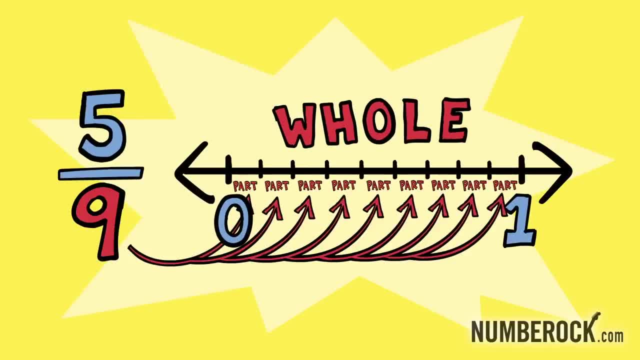 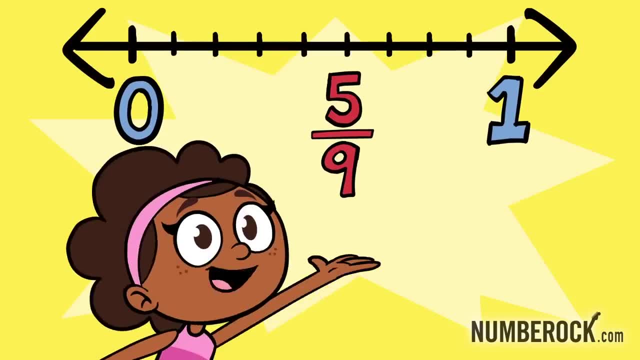 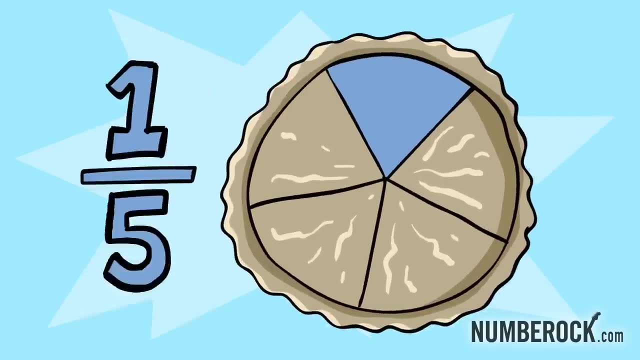 the denominator tells us into how many parts make a line that starts from zero to the fifth mark, and five nights is what you'll find when you get that far. let's use the number line to describe this pie. first, count the total pieces: there are five, five's, the denominator, all the parts. 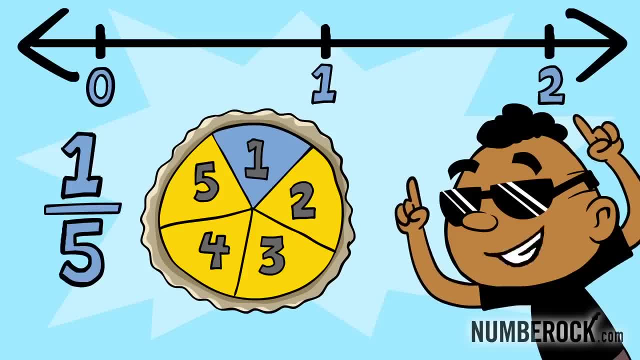 so five goes underneath the fraction bar. this number line goes from zero to two, but the fraction's less than one. so here's what to do: make five equal to one and then divide by two. make five equal to one and then divide by two. make five equal to one and then divide by two.